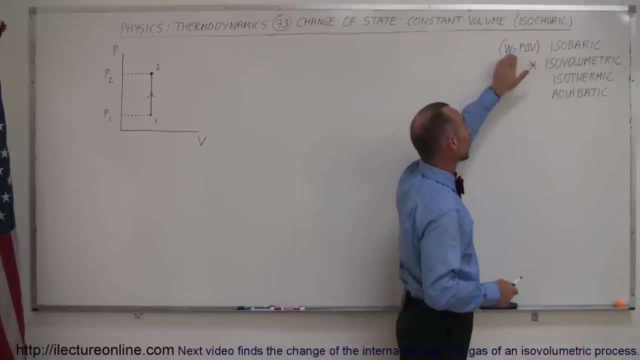 special about it. Well, in the case of an isobaric process, the work is always equal to the pressure times, the change in the volume. Easy to remember. For an isovolumetric pressure it's something different. Take a look here on the PV diagram and notice that it's a process where we go from one 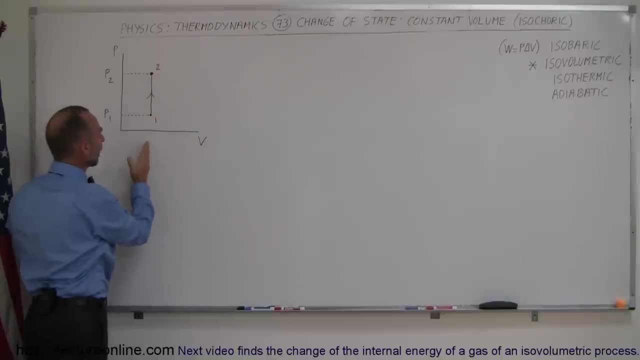 state of the gas to another state of the gas. Notice that in this case the volume doesn't change, So we can say that V1 equals V2.. It's a constant, doesn't change, And the pressure does change from pressure one to pressure two. 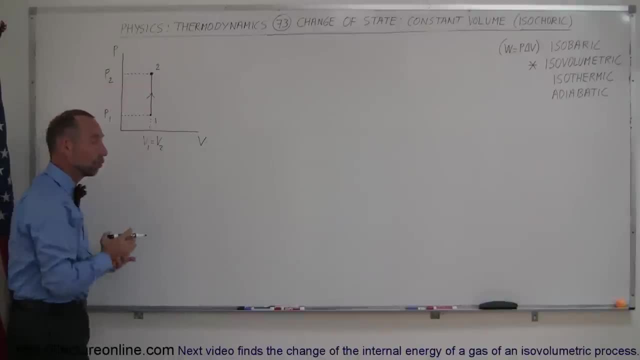 But notice here: if I asked you to find the area underneath that curve, what would you say? it is? You realize. well, the area underneath a vertical line is simply zero, And since the work done is equal to the area underneath a curve, and since there's no area underneath that curve, work done. 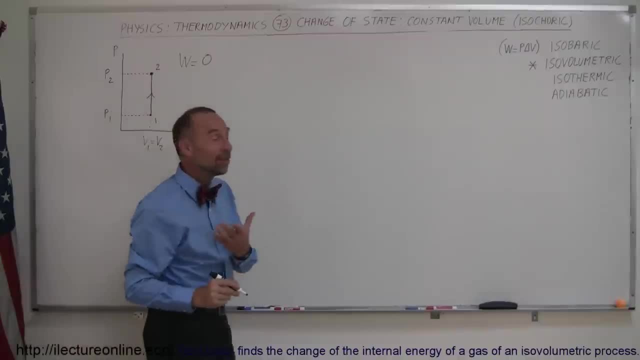 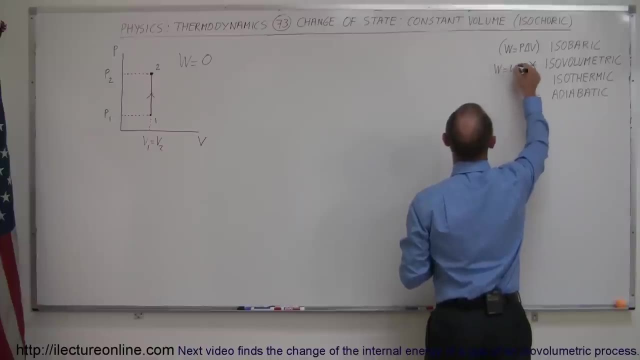 equals zero, And that's the identifying characteristic of an isovolumetric process or an isochoric process, where the work done is equal to the area underneath that curve. And since the work done is equal to zero, Now that simplifies things when we start calculating the 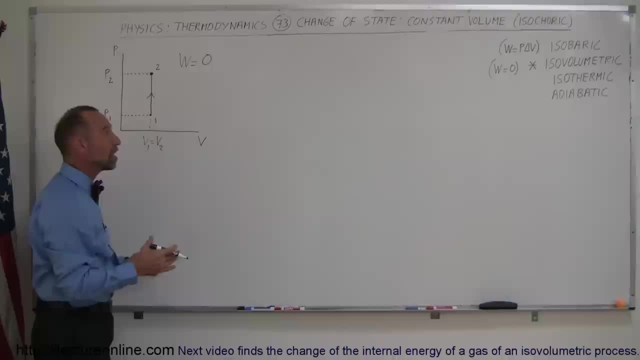 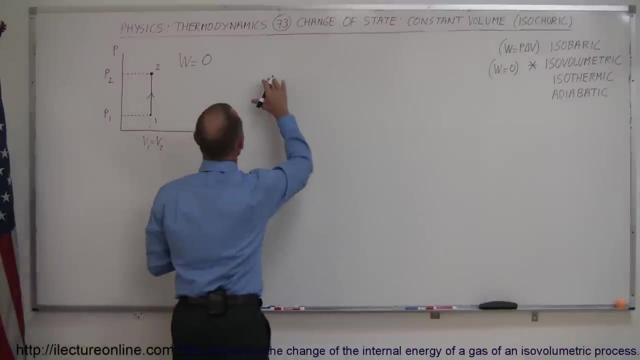 various states of the gas and how much heat is exchanged and how the internal energy of the gas changes. Because if we go back and look at the thermodynamic equation of the first law of thermodynamics, we can say that the change in internal energy is equal to the heat added to the 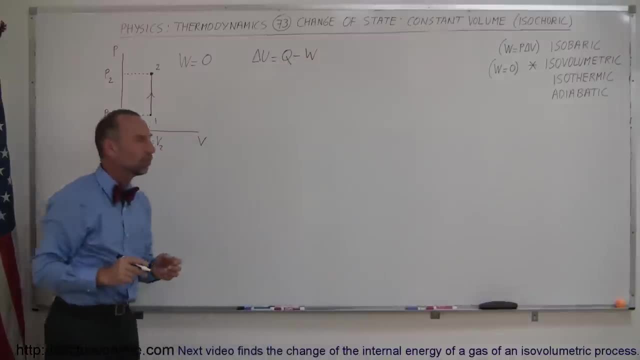 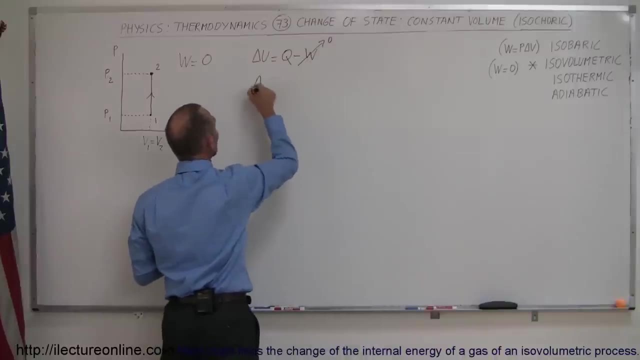 gas minus the work done by the gas. But since we know that the work done by the gas is equal to zero, the equation for the thermal energy equation is equal to zero. And since the work done by the gas is equal to zero and simplifies to the change in internal energy, is equal to the heat added to the gas. so what's? 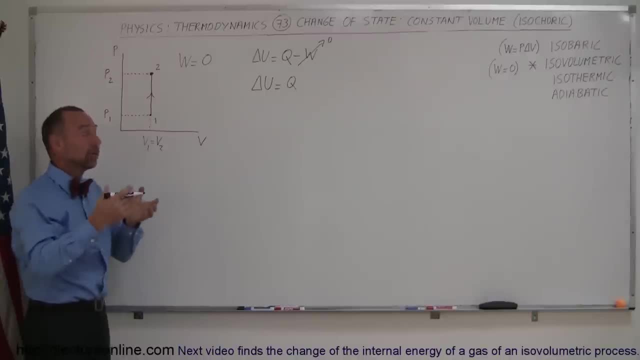 happening here is: we add heat to the gas, the gas increases internal energy by the exact same quantity. we take heat away from the gas, the internal energy of the gas decreases by the exact same quantity. now i don't know if you remember what the equation is for the change in internal 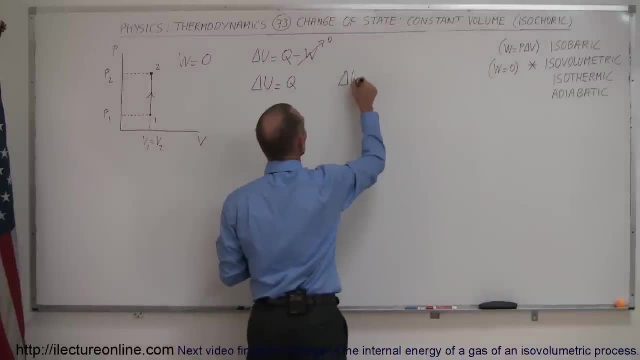 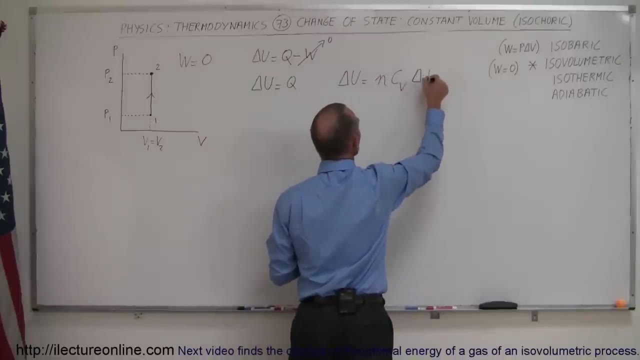 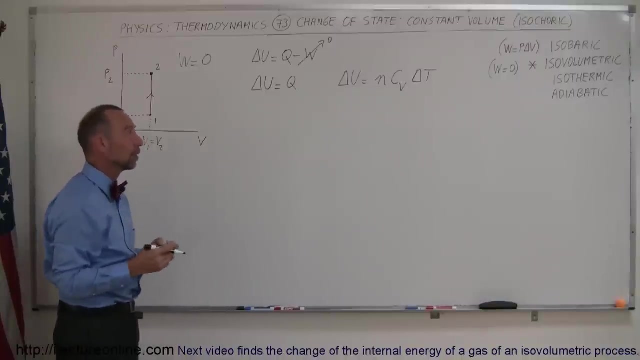 energy. but if you think back on one of the previous videos, we showed you that the change in internal energy is always equal to n, c, sub v, delta t and, of course, if delta u is equal to that, then q has to be equal to that as well, because they're exactly equal to each other.